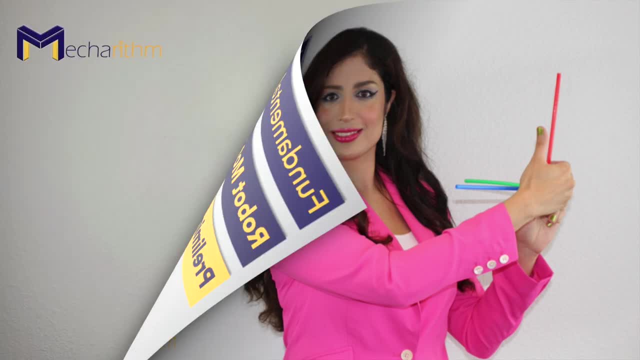 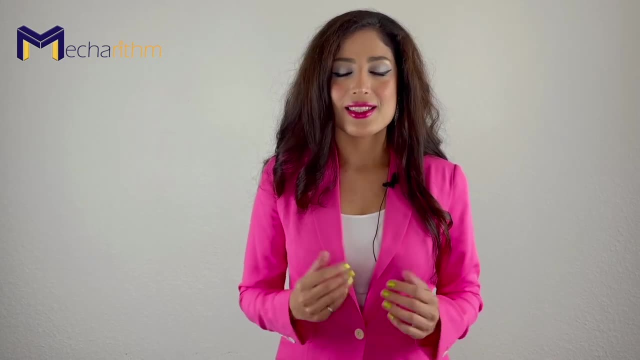 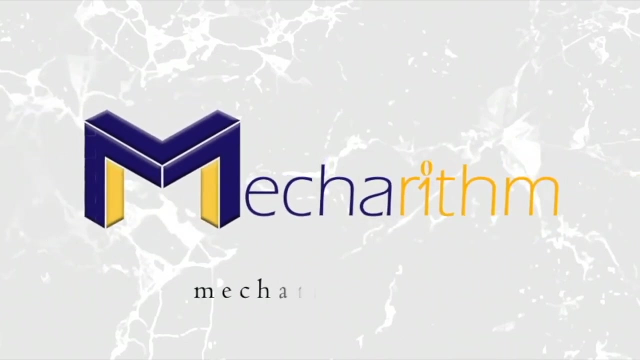 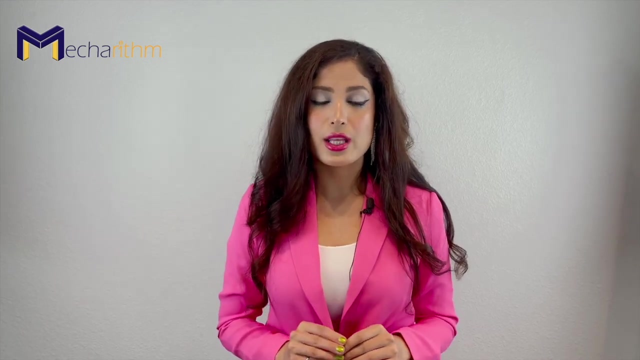 Hello everyone, Welcome to another lesson on fundamentals of robotics. This is Dr Maddy Babayasol from Mecherythm. In this lesson and a couple of future lessons, we will talk about the necessary tools needed to express robot motions. These tools are mandatory to 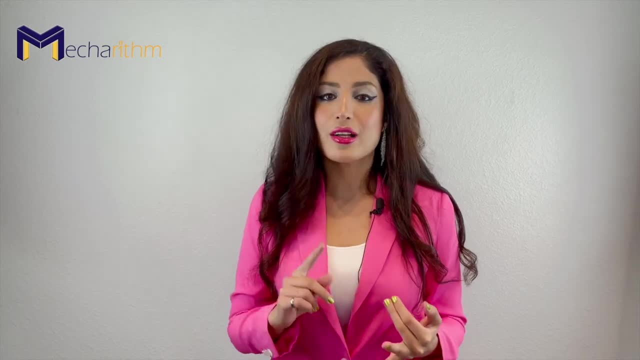 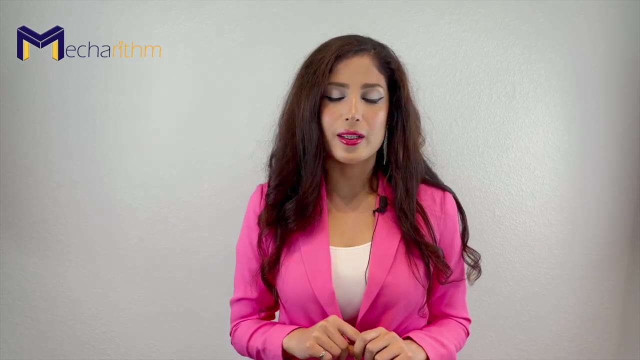 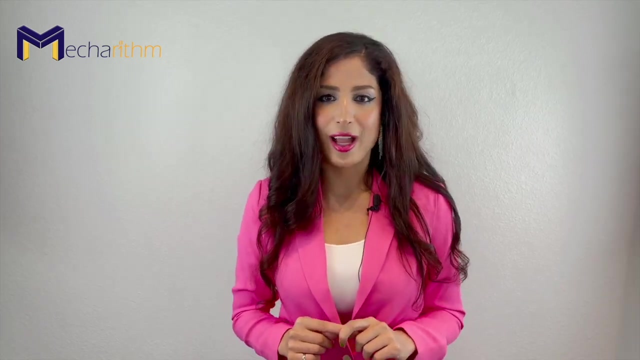 express when you want to represent the configurations, velocities and forces for robots. If you haven't done already, be sure to subscribe to our channel and follow us on social media. We'd love to have you as part of the Mecherythm family. This video has also a written version. 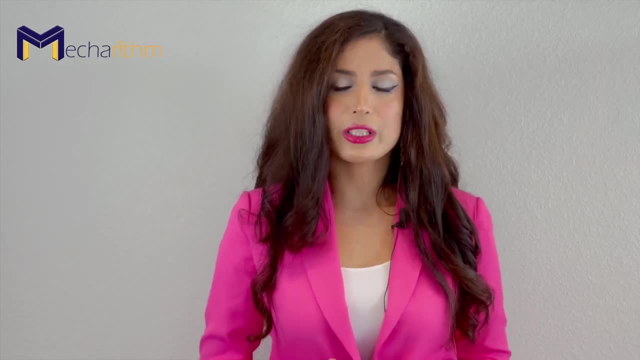 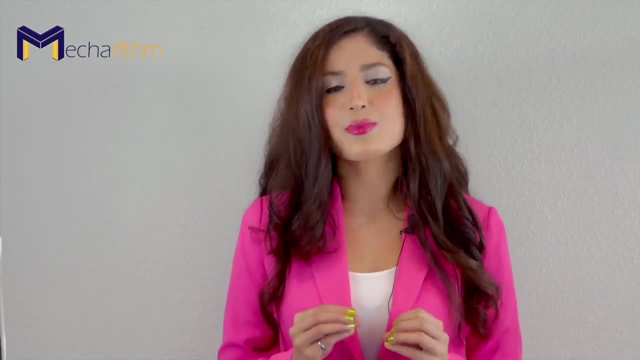 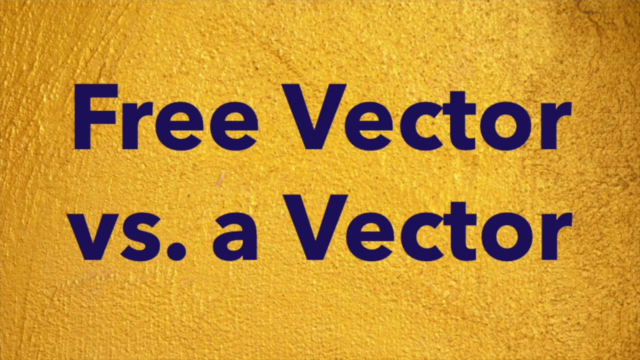 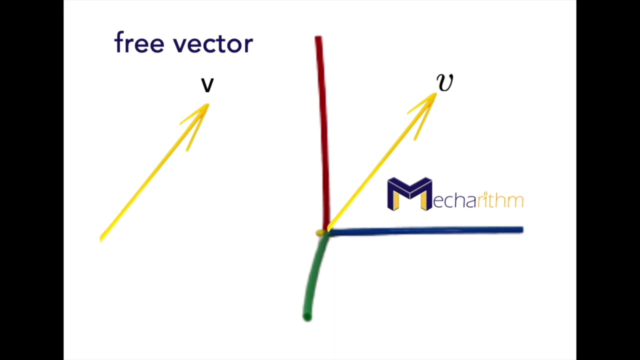 on our website. My suggestion is to watch the video first and then go read the lesson on the website. It will help you to understand and grasp the material better. So, without further ado, let's get started. A free vector is a geometric quantity and it's an arrow in our three-dimensional 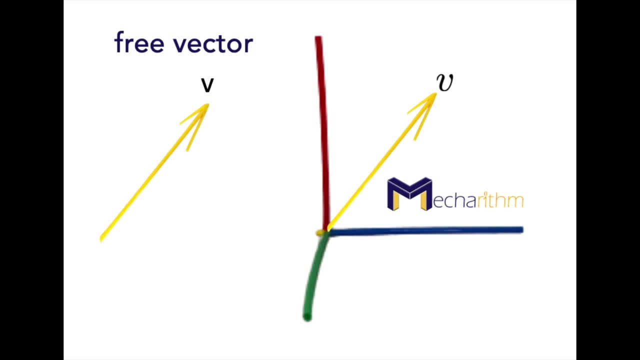 flat-space R3 that is not rooted anywhere. It has a length and a direction. A free vector is a geometric quantity and it's an arrow in our three-dimensional flat-space. R3 that is not rooted anywhere. It has a length and a direction. 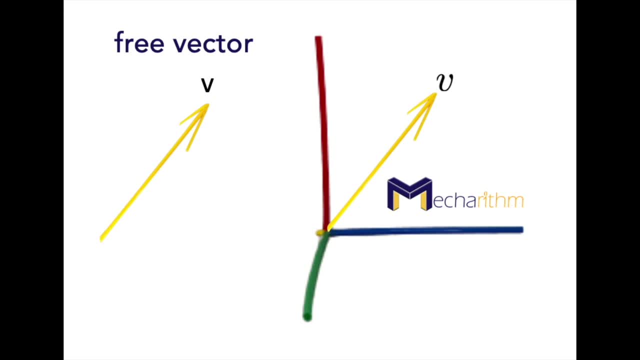 Within R3, a free vector is represented by the capital V. A vector is linked to the Roman word pauve, which meansр A relación between independent force and shells, allowing it to be defined through linking Land and Earth. here, In robotics, a free vector is denoted by the capital V. A vector, on the other hand, is: 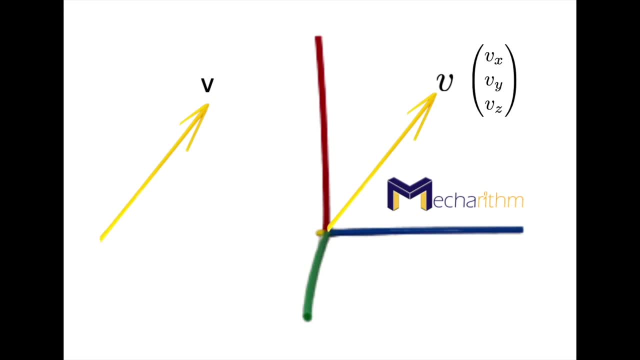 the same as free vector, but it's expressed, with its coordinates, in a reference frame and length scale chosen for the space. OK, just a few words about a free vector, whether you have interesting examples for yourself. in this case, In robotics, vectors are represented by an italic letter V in R3.. A vector is dependent. 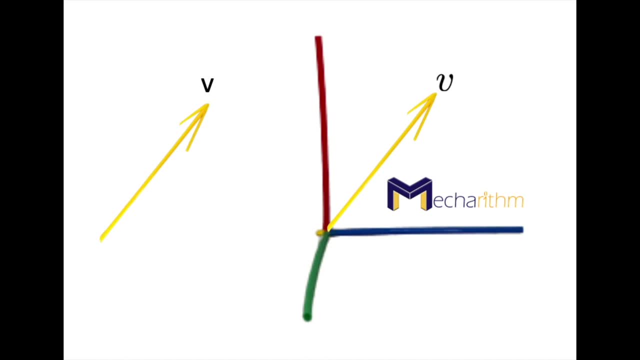 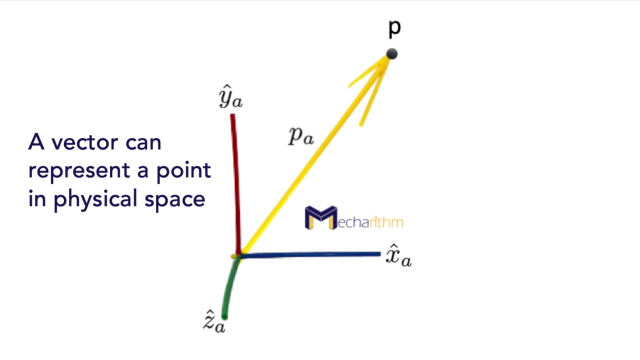 on the choice of the coordinate frame and length scale, whereas the underlying reference free vector is unchanged by choice of the coordinate frame or the length scale. In other words, the free vector is coordinate-free whereas the vector is coordinate-dependent. A vector can also represent the point P in the physical space. 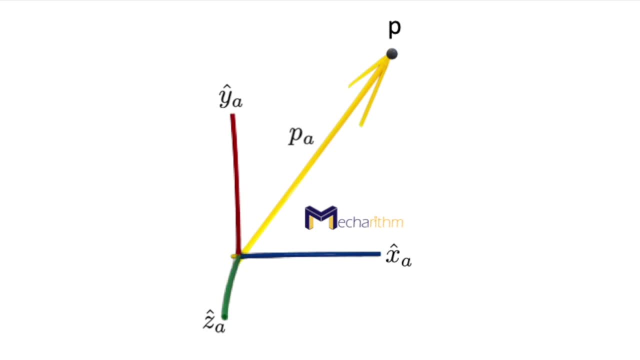 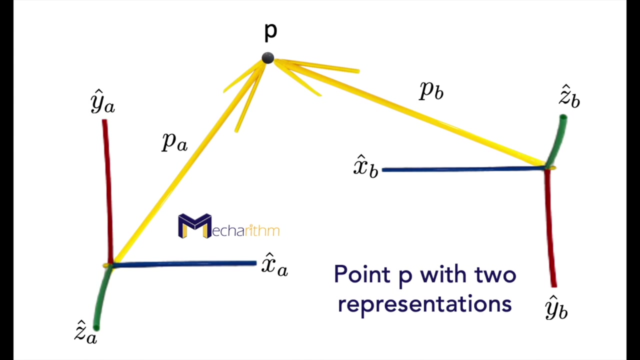 If we choose to give this physical space a reference frame and a length scale, the point is a vector from the origin of this reference frame to the point. It's then represented as an italic P. in that space, The same point has a different representation by changing the length scale and the reference. 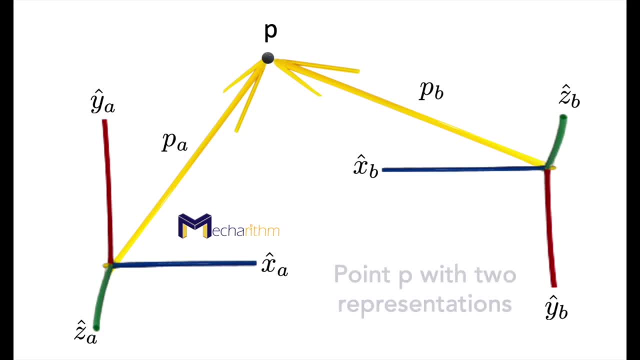 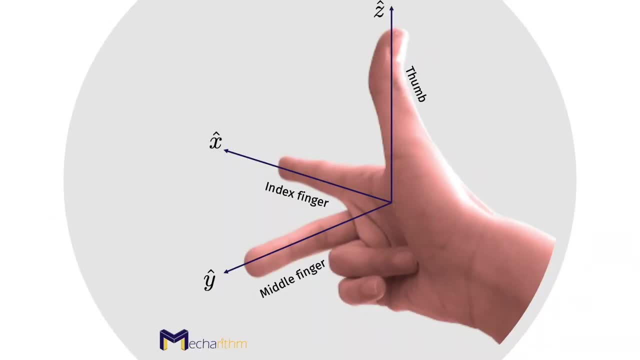 frame. as you can see in this figure, In robotics frames are important. We use frames to represent the robot's configurations, velocities and forces causing the motion. Frames in robotics have an origin. They consist of orthogonal X, Y and Z coordinate axes and they are right-handed. 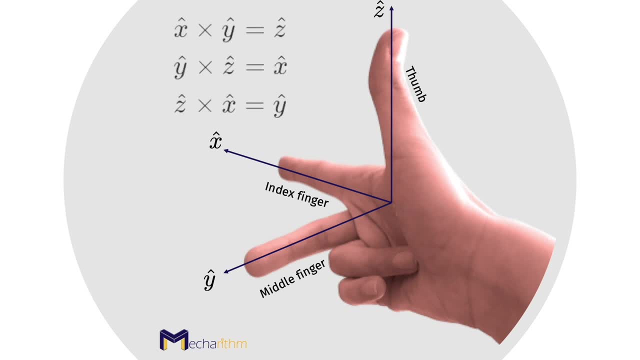 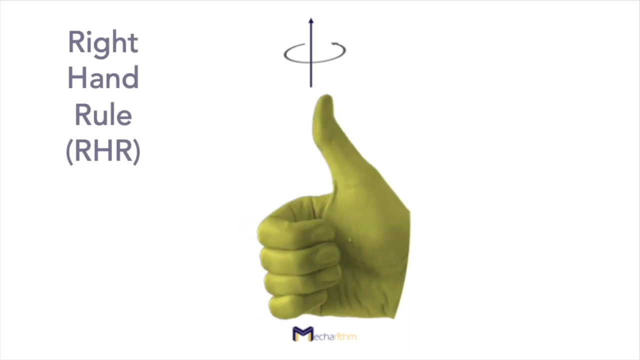 They are not vertical, And this means that the cross-product of the X and Y axes is Z and so on. They are stationary, And this is from Newton's laws that the reference frames are always considered to be inertial. Positive rotation about an axis follows the right-hand rule. 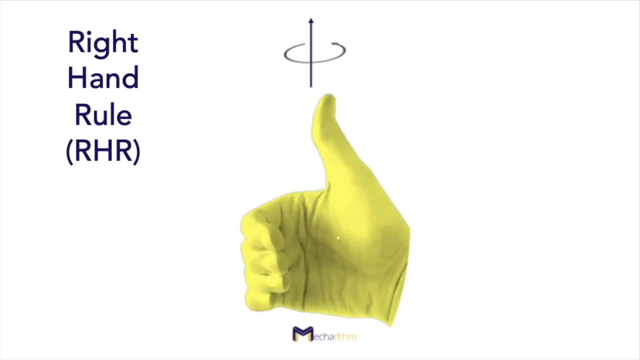 If you align your thumb with the axis of rotation, then the positive rotation follows the right-hand rule. If you align your thumb with the axis of rotation, then the positive rotation follows the right-hand rule And the positive rotation is in the direction that the finger curls, as you see in this. 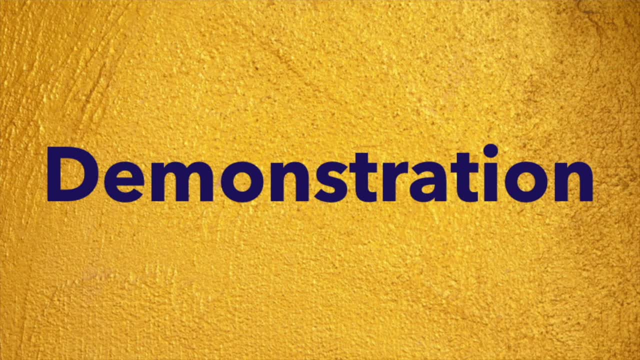 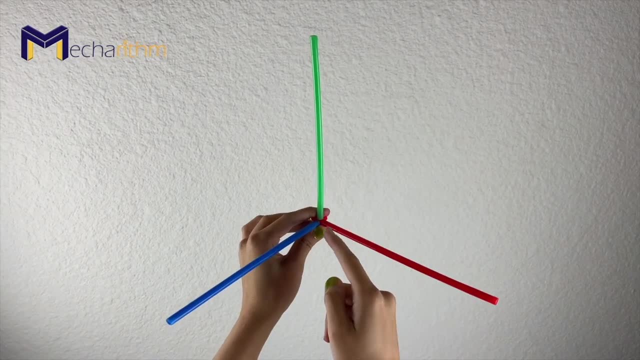 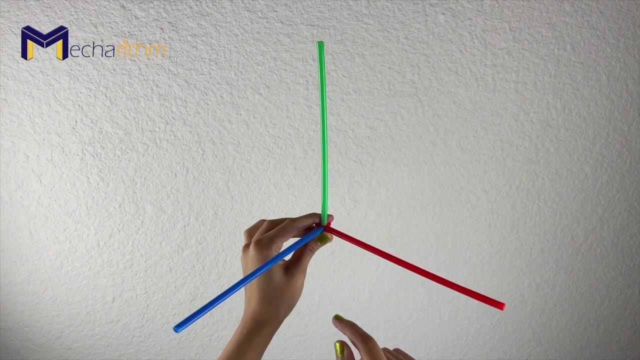 animation. In order to conclude this lesson, I want to show you a simple demonstration. Suppose that this is a coordinate frame attached to a robot joint. I want to show the positive rotation around X, Y and Z directions. So this is the X direction. 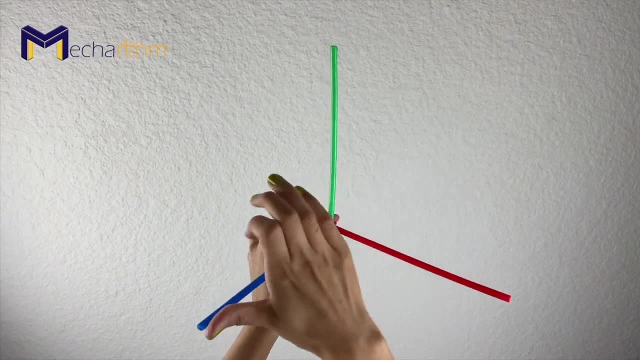 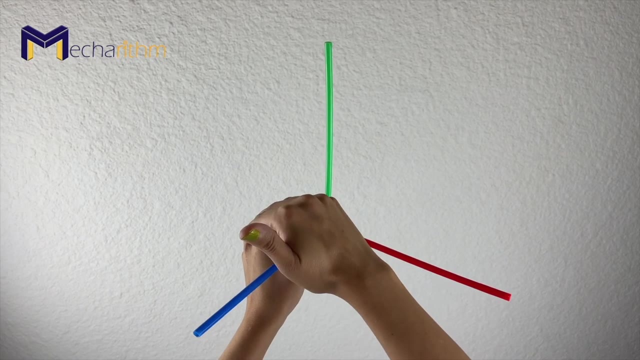 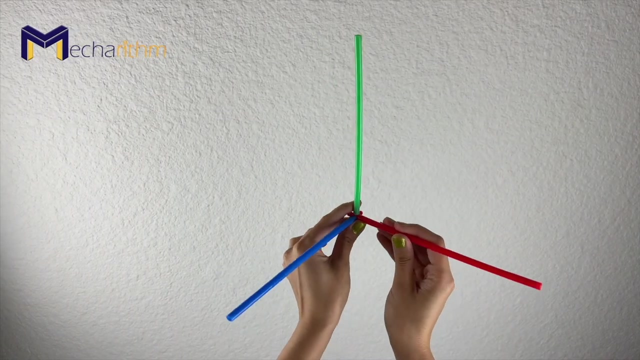 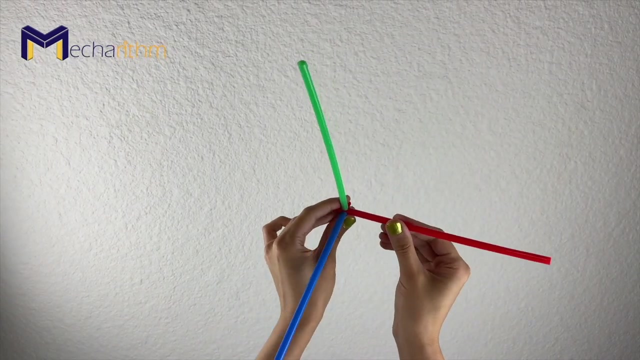 positive rotation around the x-direction would be when my sum is in the direction of the axis, the curling fingers show the positive rotation. so this would be the positive rotation around this x-axis. the positive rotation around the y-axis would be in this direction. so it would be in this direction and the positive